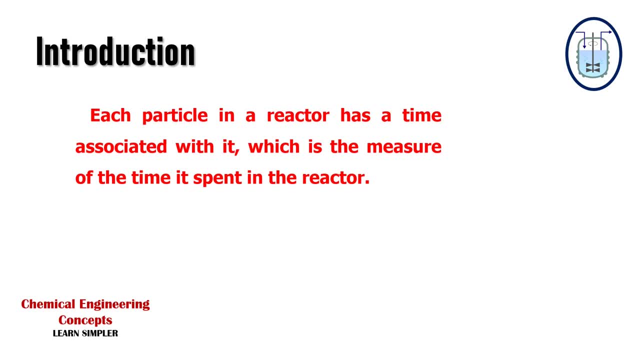 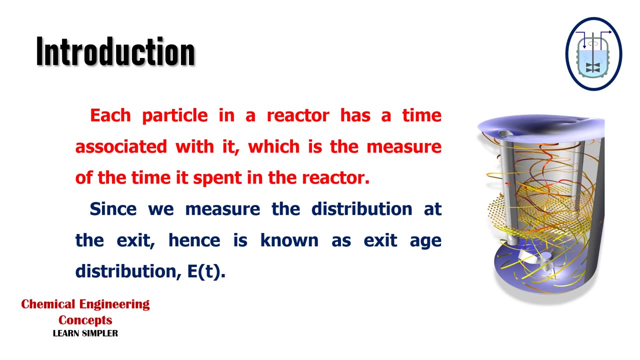 residence time of the atoms inside the reactor. This is general, non-ideal patterns that you can see here, Right. So, since we measure this distribution of time of all the atoms at the exit of the reactor, that's why we call it as the exit age distribution. 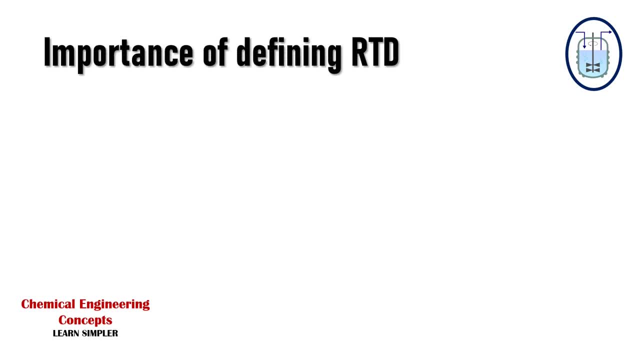 Now, guys, we should know the importance of this RTD. Okay, To feel the importance of the RTD, we know about the ideal. That means that is only the real price ofacking. Now, for instance, we can, I gives you a bath. This is called the wichtiger point here. Let's. 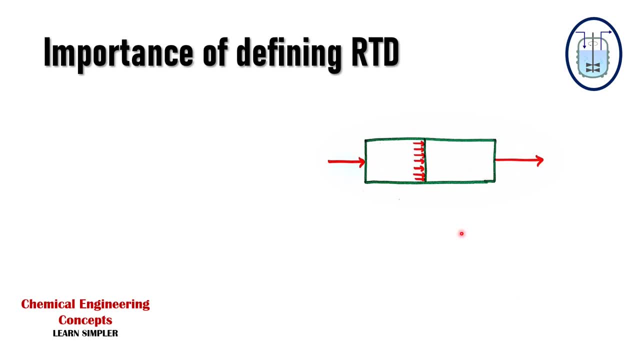 think about RTD. OK, So in this project we need to compare the Long-circuit space and the long-circuit Fucking of these atoms, and we 라고 at which the there will be infinite mixing in the radial direction and the 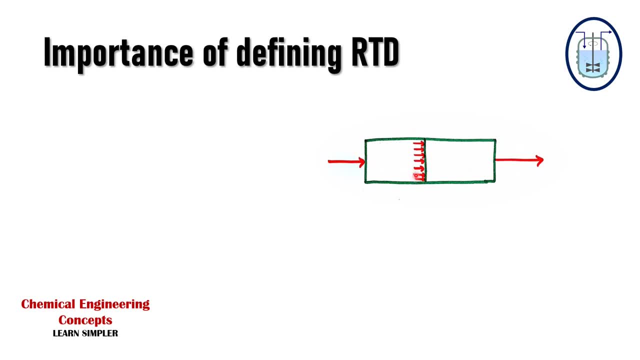 and there is no mixing, no back mixing, in the axial direction, or we can say the longitudinal direction. so, guys, there is a flat velocity profile in a PFR. so when I am talking about the non idealities in an, in an PFR, that's what I 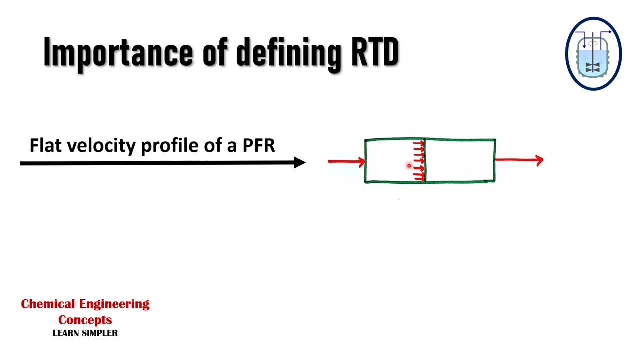 mean that there will be a deviation from the laminar flow. okay, you should understand that for the PFR there is a important assumption that we have a laminar flow. in all other types of reactor, the various atoms in the feed spent different times inside the reactor, that is, there is a distribution of 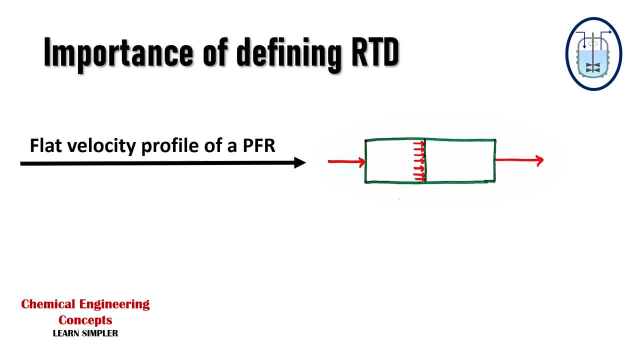 residence times of the materials within the reactors. let's take an example of a mixed flow reactor. now we have a mixed flow reactor. yes, this is a mixed flow reactor, okay, so some of the atoms entering the CSTR- we call it also as the continuous stored tank reactor. so 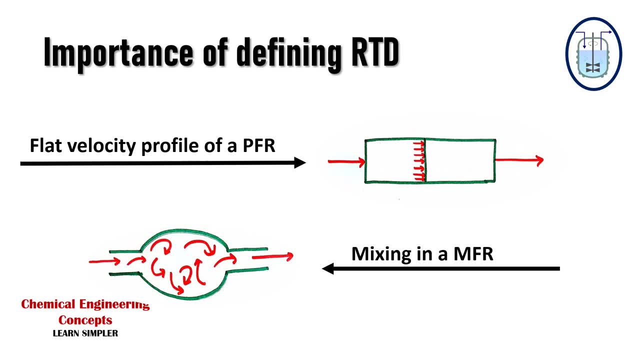 some of the atoms entering this MFR leaves it almost immediately because material is being continuously withdrawn from the reactor. other atoms remain in the reactor almost forever because all the material is never removed from the reactor at one time and many of the atoms, of course, leave the reactor after spending a 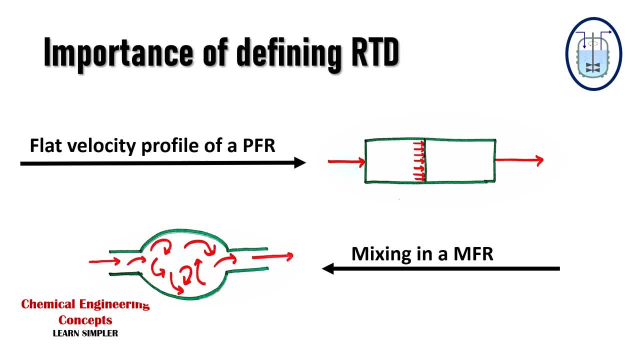 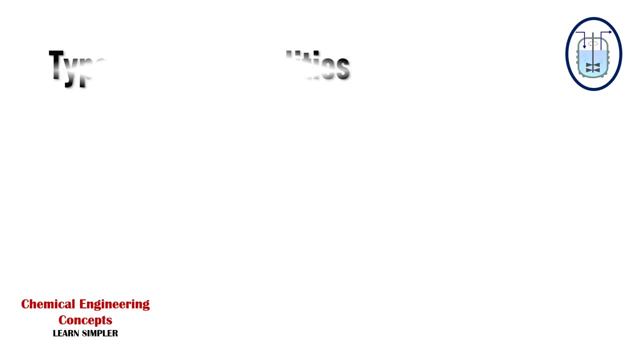 period of time somewhere in the vicinity of the mean residence time. okay, so this is how important to understand the history of the molecules or atoms inside the reactor. that is the residence time distribution. so, guys, these are the type of non-idealities okay, when they are, there is. 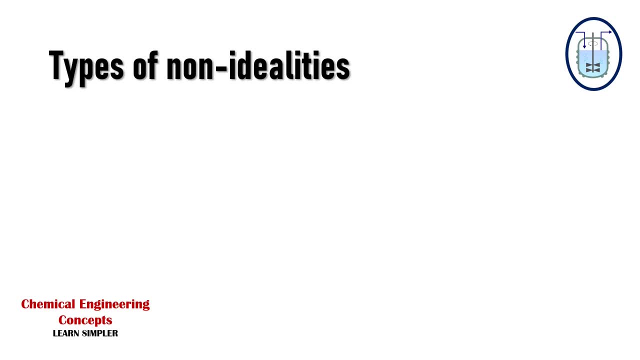 a deviation from the ideality. there must be some non-idealities and today we will be exploring them. we have PFR. okay, so in PFR generally, if I saw, if I call as the ideal PFR, that means we will be having no axial mixing and, if any, back mixing. 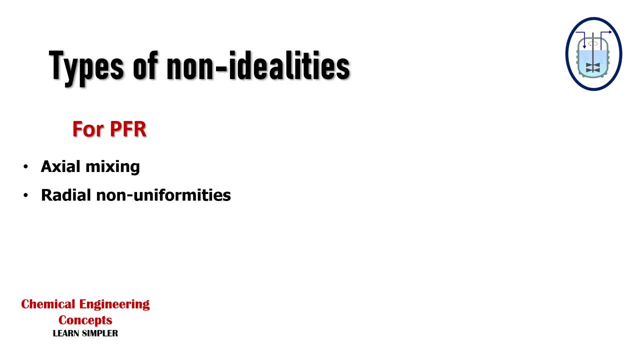 is introduced. that is the non-ideality we also want. radially, everything is to be uniformed in a PFR. okay, the concentration has to be uniform. but if there are non-uniformities in the concentration, that's what we call as the non-ideality as well- there could be dead. 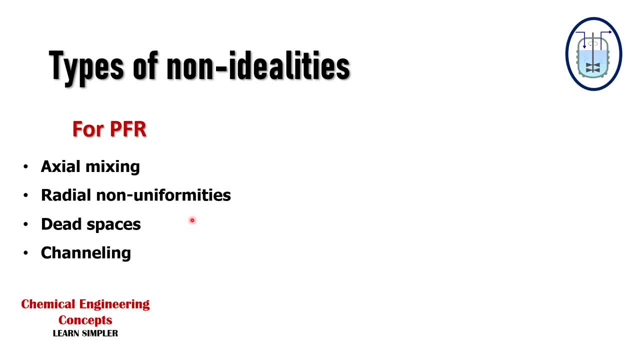 spaces in the corners, okay, or in the lower part of the tubular reactor. and we can also have channeling inside a PFR. we also can have the MFR- okay, there could be non-idealities in the MFR as well. so dead zones are there in an MFR. recirculation is there? 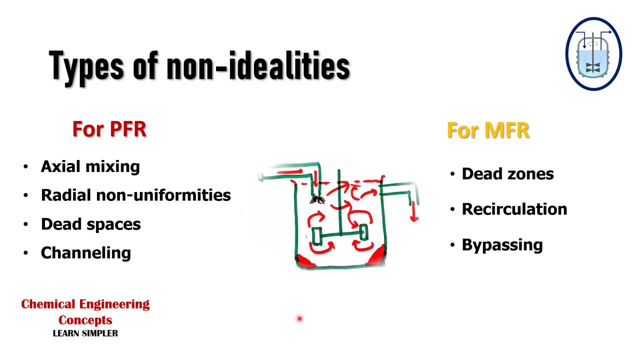 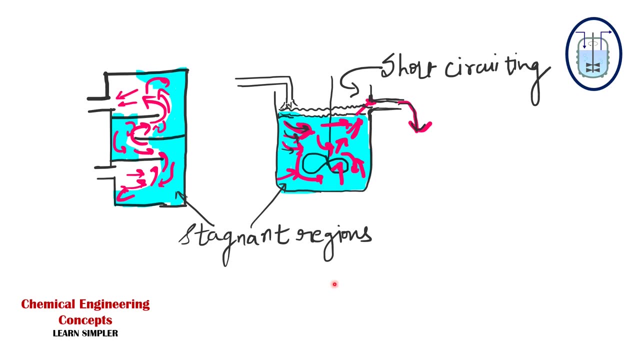 in an MFR and there could be bypassing in an MFR. okay, so these are the common non-idealities related to the mixed flow reactor. you can see all of them here. now you can see the deviation from the two ideal flow patterns. okay, so we have these two types. 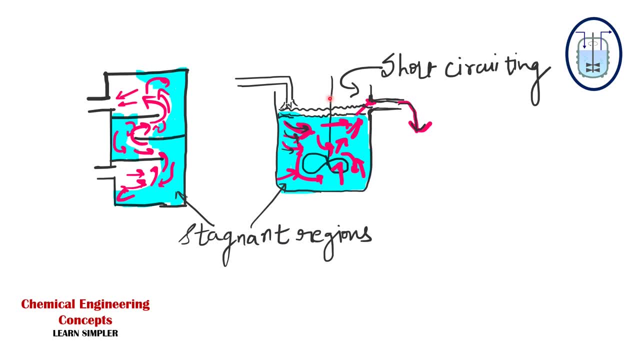 reactor arrangements. okay. so deviation from the two ideal flow patterns can be caused by channeling of the fluid and we can see, okay, and the deviation can be because of the recycling of the fluid or by the creation of stagnant region in the vessel. okay, so we can have these type of stagnant region in the corners. 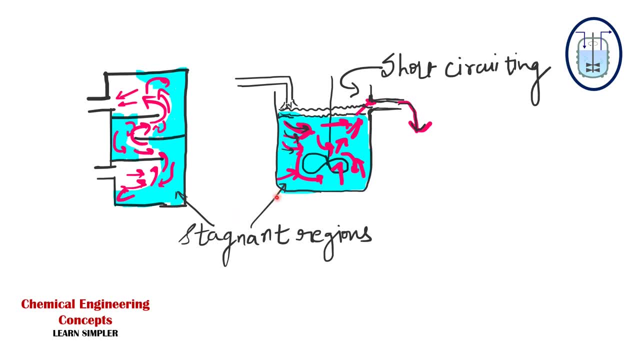 okay, where the reactant comes and get trapped and will not be allowed forever, maybe, maybe, forever, to go outside, outside the reactor, right? so, guys, in all these types of process equipment, such as heat exchanger, pegged columns and reactor types, there could be many type of reactors, so this type of flow should. 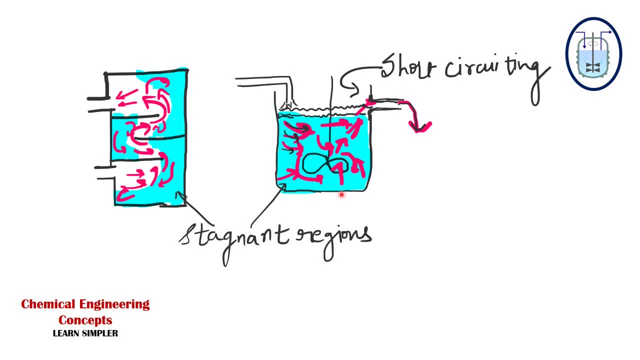 be avoided because it creates non-idealities, since it always lowers the performance of the flow of the liquid. so it creates non-idealities of the unit. okay, so we can say: you can see the short circuiting as well, the reactant coming and just going outside, we know, without being reacted inside the 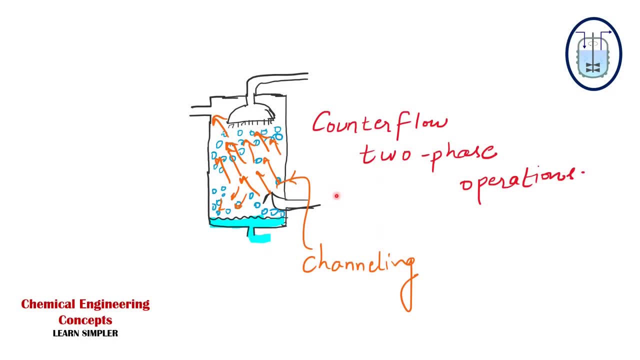 reactor. you can see one more non-idealities in a counter flow to phase operation. okay, so you can see a counter flow to phase operation in which we can observe a channeling. okay, so you can see the liquid bubbles. these are the liquid bubbles and this is is in orange. you. 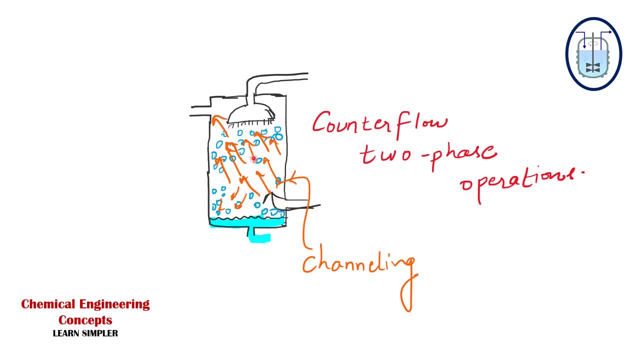 can see the air, the air will go, air will come and just without being completely attached or we can say completely reacted, or being phase transfer between the liquid, it will go out. outside this, this column right, so you can see these Types of Non-Idealities. AiB labeling: available selling number: Flow aprender. 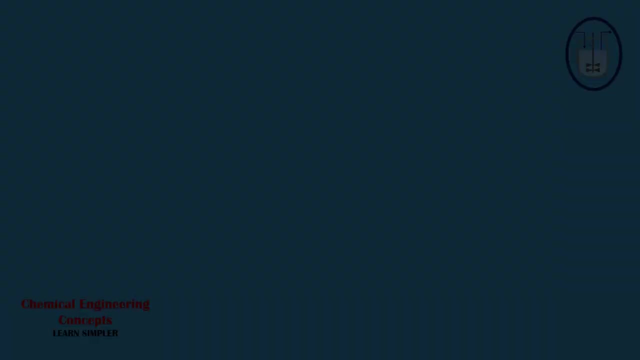 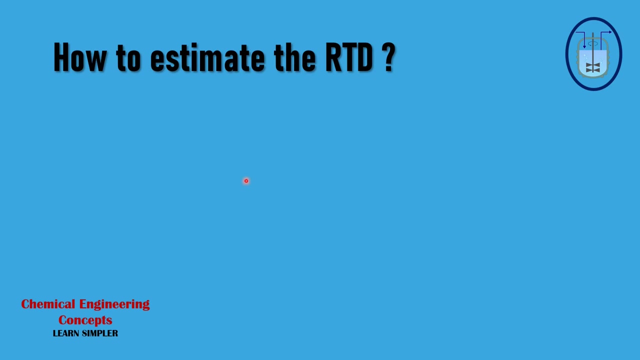 間 can come inside the process equipment right. so how to estimate the rtd? this is a very big question, guys. we have various equipments and we want to measure the history- okay, the time history- of all the molecules inside the reactor. so there could be a very important method, which is the stimulus. 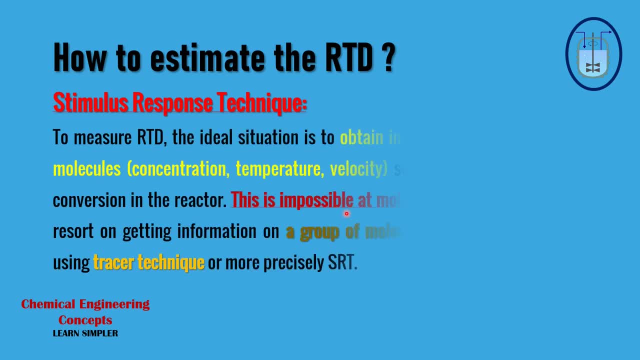 response technique. that is in which what we are going to do now to measure this rtd, what we are going to do actually, the ideal situation is what ideal situation is? to obtain the information on each and every molecule. what information? the information about the concentration, time, temperature, sorry- and the velocity of each and every molecule. okay, so we can calculate. 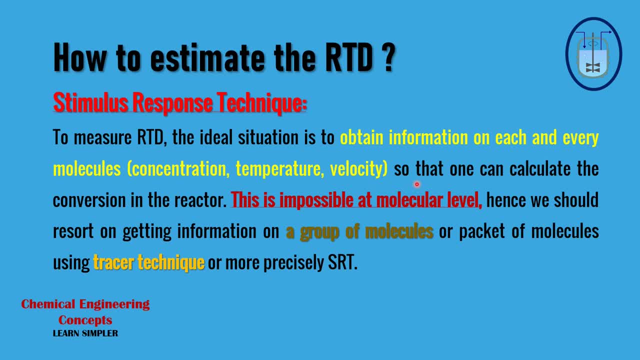 the conversion inside the reactor. now, as we know this data, to look at each and every molecule, it is next to impossible because we are dealing with large reactors. hence we should resort on getting information on a group of molecules. okay, we will here choose a volume and we will measure the changes across that volume. so 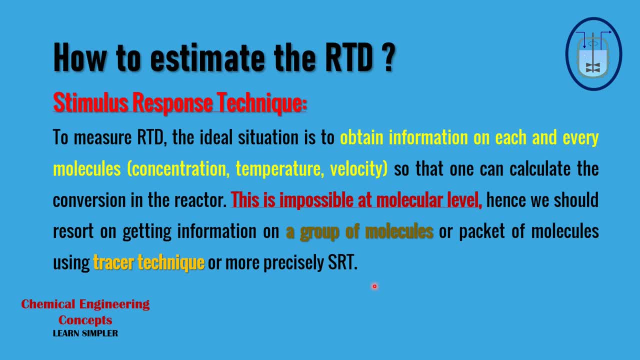 there has to be a control volume here. okay, we also call it as a packet of molecules and we will use tracer technique, or we precisely call it as the stimulus response technique. in the tracer technique, what we will do, we will insert some different foreign material inside our reactor and we see the when we when it will come out of the reactor, what, 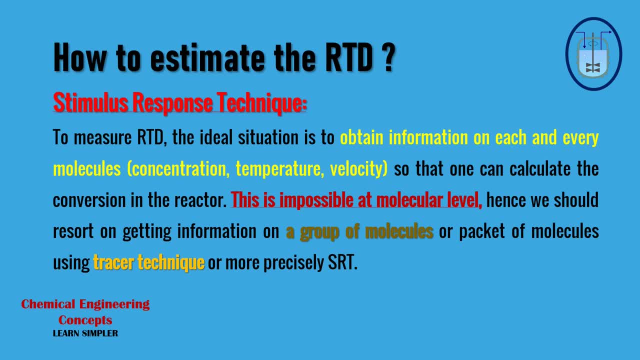 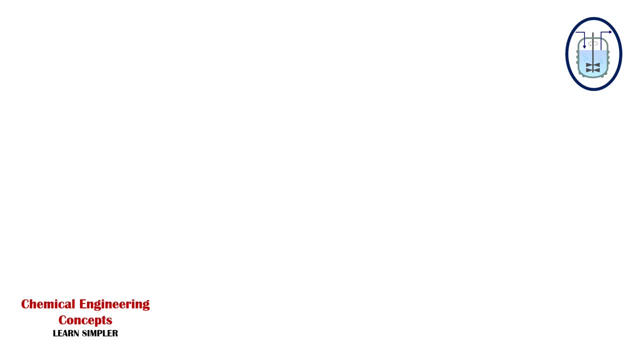 pattern does it follows okay. so here we see, we can like measure the residence time distribution inside the reactor. so the RTD is determined experimentally by injecting an inert material, which we are calling as the tracer, into the reactor at any time t equal to zero. so how these stimulus response technique works, and at 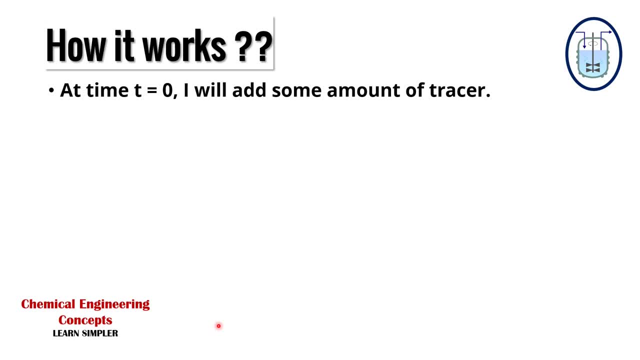 TMT equal to zero, I will add some amount of tracer and then in measuring the concentration C in the influent stream as a function of time. okay, this is our simple technique. this is our reactor, which is a real vessel, as you can see that we are. 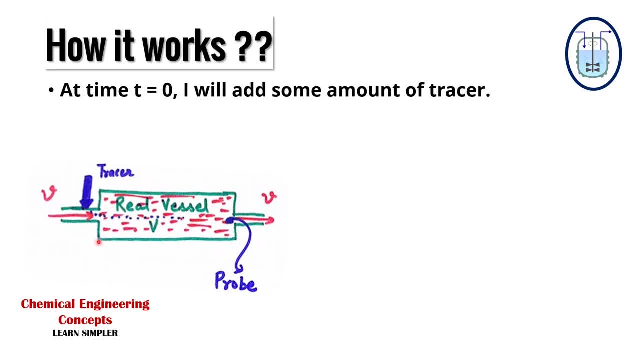 measuring here about. we are taking here the PFR. you can see the PFR: right, there is a tracer which is injected at the inlet right and we have a probe at the outlet that will measure the exit stream. okay, and this effluent, effluent of the, 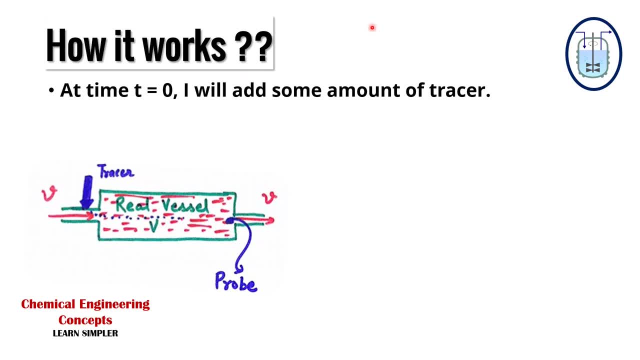 tracer will be measured at the outlet. okay, this is what we have now. in addition to being a non reactive species, these are the basic qualities of there there are. there are basic qualities of this: tracer amount, tracer element. okay, so this has to be a non reactive species that is easily detectable. this tracer, 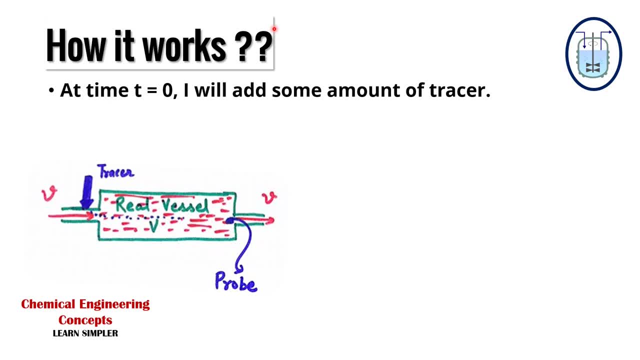 material should have physical properties very similar to those of the reacting mixture and it should be completely soluble in the mixture guys. these are the important properties that you can write. it should also not absorb on the walls or other surface inside the reactor. these are the basic properties of a tracer. more preferably it could be a colored and radioactive. 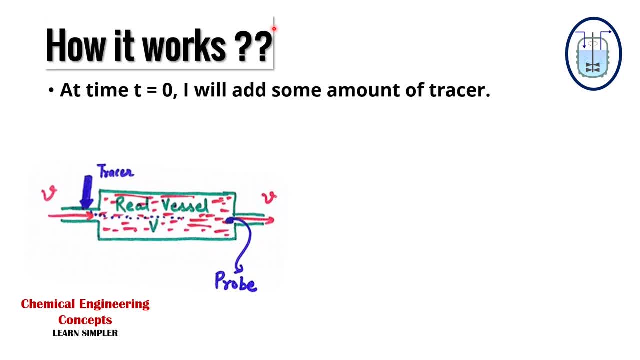 material. along with there could be inert gases. okay, which are the common examples to be used as tracer material? the two most used methods of injection are pulse input and the step input, and what you are watching here is simply the pulse input. the effluent concentration versus time curve is referred to as the C curve. okay, guys. 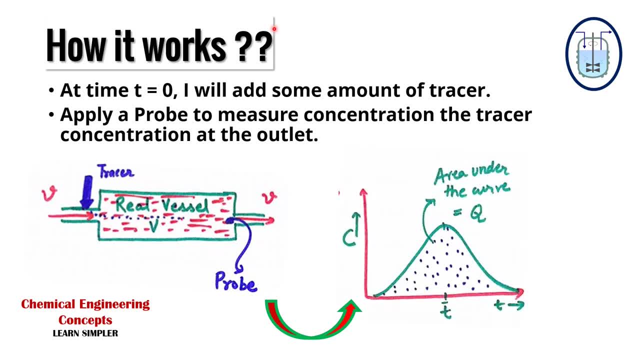 you can see a C curve here. this is what we will be getting. after the RTD analysis, we shall analyze the injection of a tracer pulse for a single input and single output, a system in which only flow and not the dispersion carries the tracer material. okay, so there will be no back mixing. 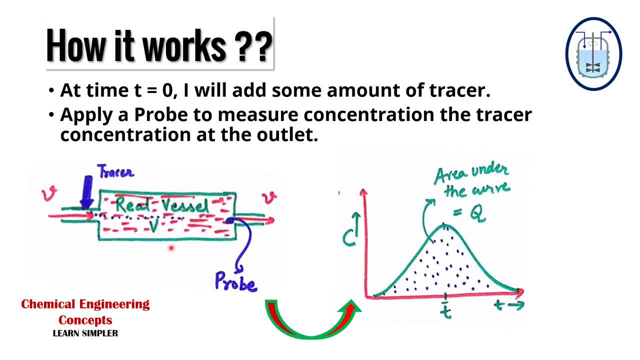 I already told you that we are supposing it to be a PFR. so we are assuming that there will be no dispersion and we will measure the tracer and we will have the movement of the tracer material just because of the flow. okay, so only flow carries the tracer material across. 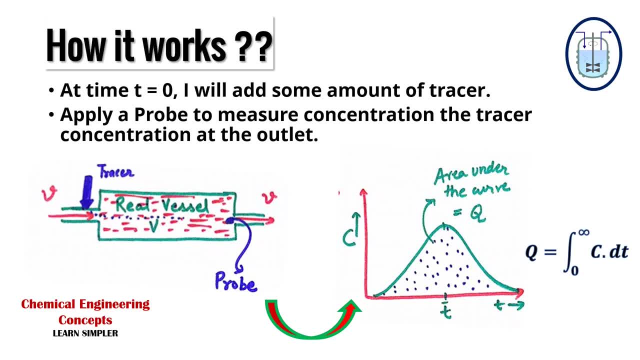 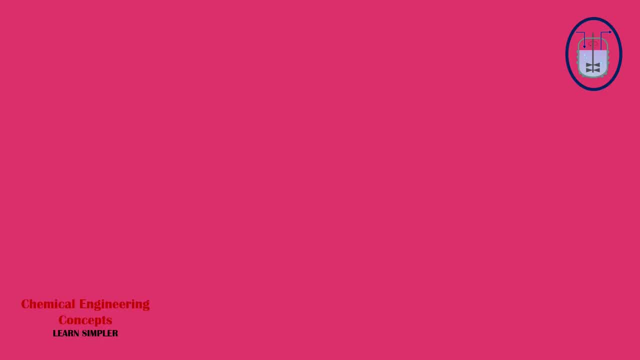 the system boundaries. this is how the stimulus response technique will work, and Q is the flow rate that we will get at the outlet. now it's an understood thing that a fluid taking different routes through the reactor and so take different lengths of time to pass through the vessel. the distribution of these times for the 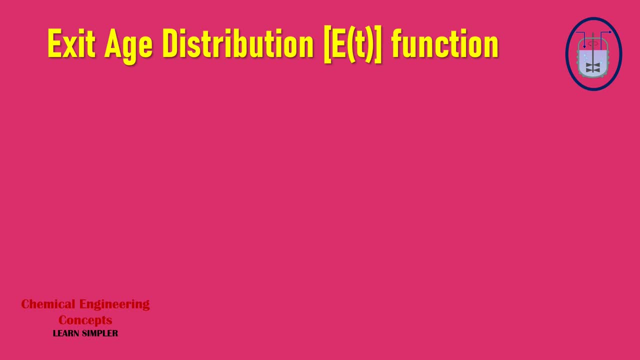 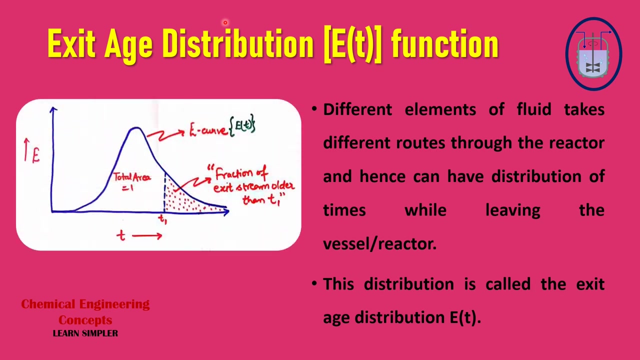 stream of the fluid leaving the vessel is called the exit age distribution, which is represented by ET. okay, or we can call it as the residence time distribution, RTD- of the fluid. it has a unit of time inverse, so we have different things related to the exit age distribution that you can see here: the 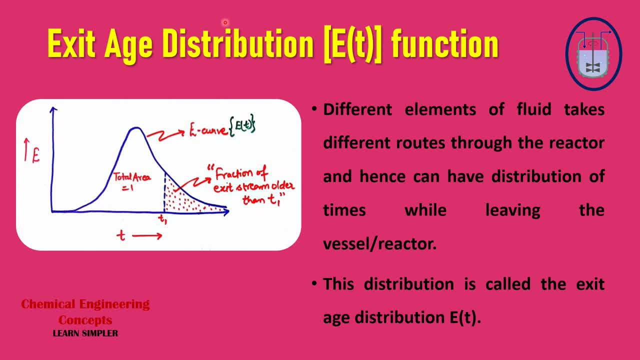 total area under this E curve is obviously one, then that we will prove further. and if I talk about some fraction, okay, if I talk about some fraction, anything, if you call anything at time, t equal to one. so from this point till the end of this curve, till the point where the curve 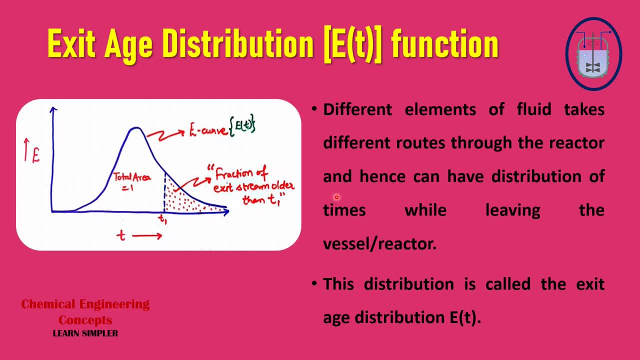 ends and touches the x-axis, that will be called as the fraction of the exit stream which is older than the time: t1. okay, you should remember these terms, how we are defining them, how we are defining the E curve and how to define the different fractions then. okay, so let's. 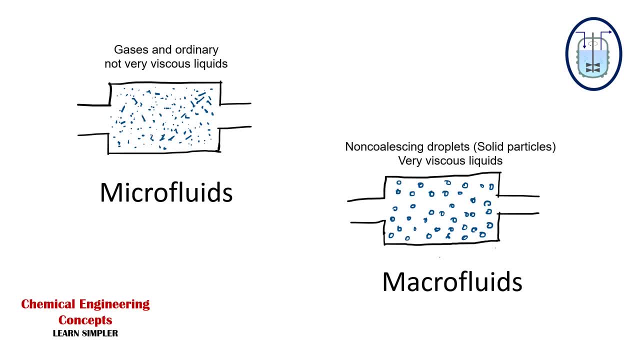 so let's look at the basic two types of fluid that we have. so first one you can see is the microfluid. okay, we can. we can see the microfluids, which are generally gases and ordinary, not very viscous liquids. in these microfluids, what? 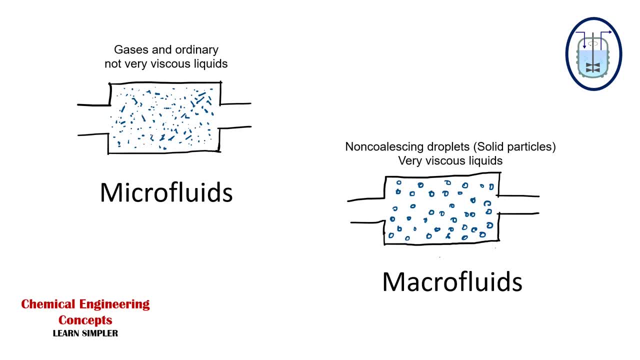 happens is that individual molecules are free to move about and intermix. and if I talk about the other type of fluid, that is, macrofluids, in the macrofluids we have non coalescing droplets, which we call as the solid particles, solid like particles, and actually they are very viscous. 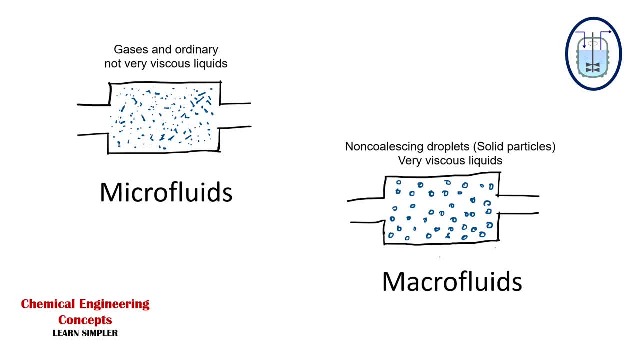 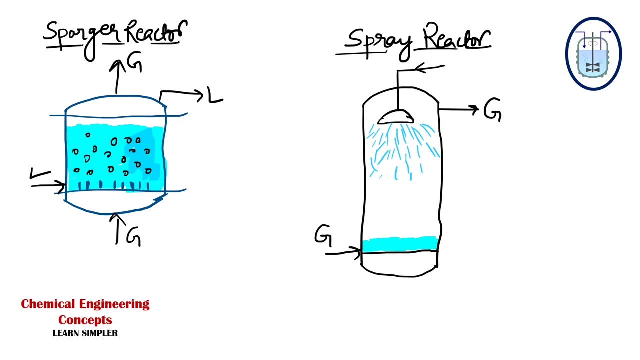 liquids. what happens in the macrofluids is that molecules are kept grouped together- okay, grouped together in some aggregates and packets. so these are the two major types of fluids that we generally deal in the reactors. now let's look at some examples of these micro and macro fluids. so, guys, let's see the two examples that we have.